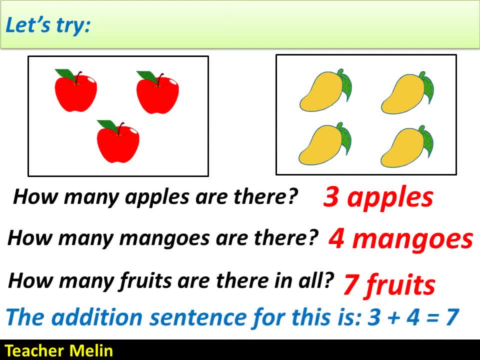 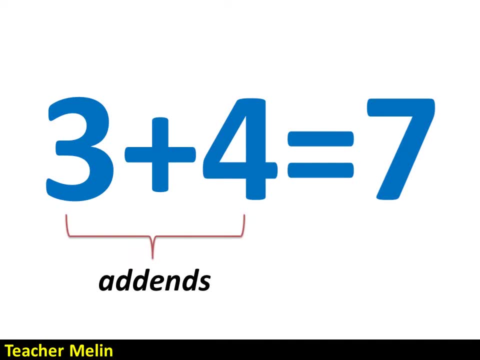 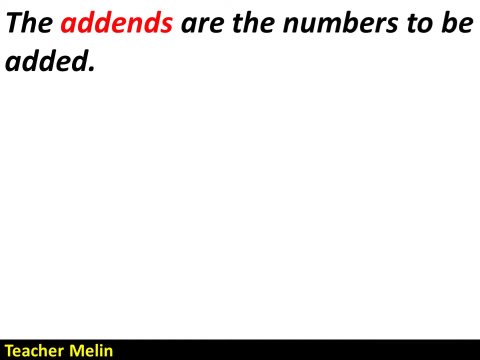 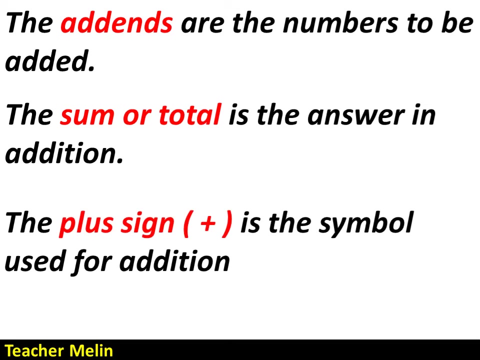 There are seven fruits. The addition sentence for this is: Three plus four equals seven. Three and four are the addends and this is the plus sign and number. seven is the sum. The addends are the numbers to be added. The sum, or total, is the answer in addition. 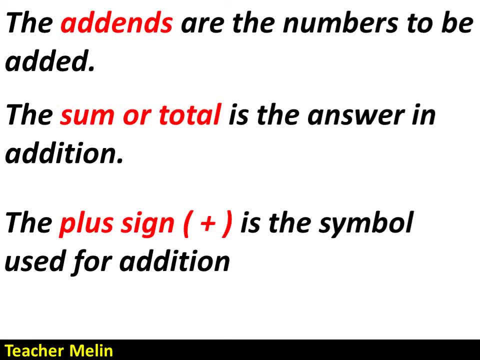 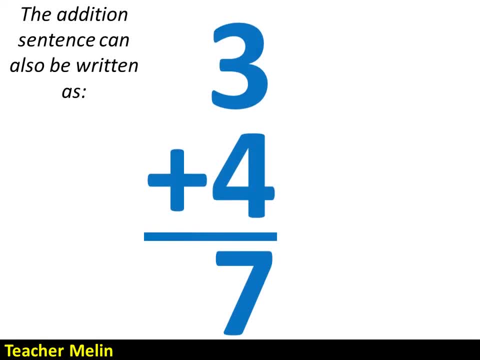 The plus sign is the sum. The number is symbol used for addition. The addition sentence can also be written as: Three plus four equals seven. Three and four are the addends, because these are the numbers to be added And this is the plus sign. 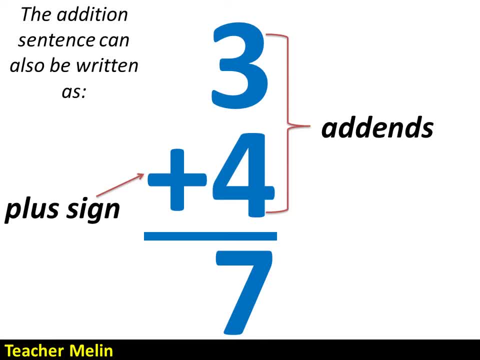 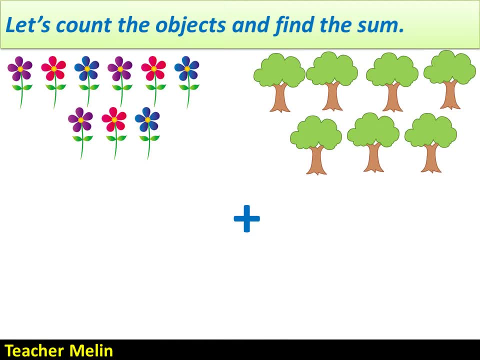 The symbol used for addition And the total, or the sum, is 7. Let's count the objects and find the sum. There are flowers and trees. Let's count the flowers: 1, 2, 3,, 4,, 5,, 6,, 7,, 8,, 9. 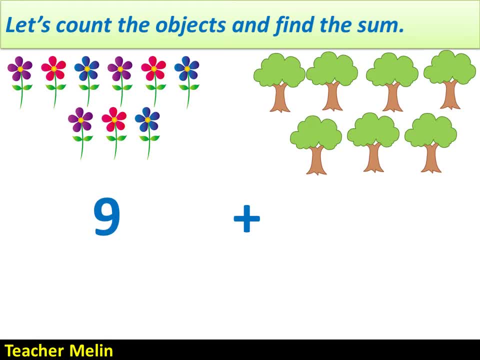 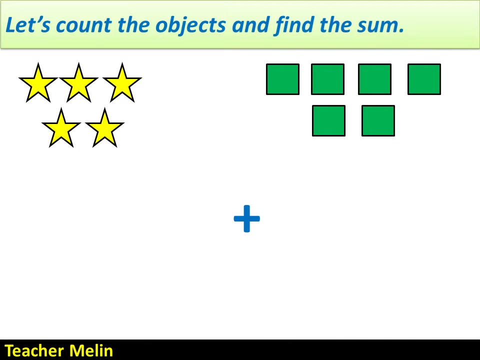 There are 9 flowers. Let's count the trees Ready: 1, 2,, 3,, 4,, 5,, 6, 7. There are 7 trees, 9 plus 7. 9 plus 7 equals 16. Another example: 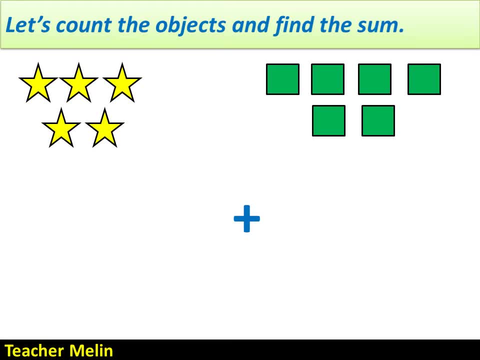 The stars and the squares. Let's count the stars and the squares. Let's count the stars 1,, 2, 3, 4, 5. There are 5 stars. Let's count the squares: 1, 2, 3, 4, 5, 6. 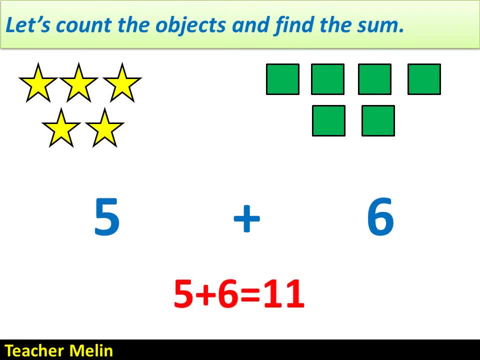 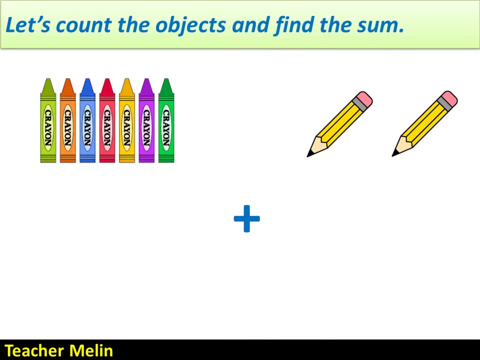 6 squares, 5 plus 6. 5 plus 6 equals 11 Crayons And pencils. Let's count the crayons: 1,, 2,, 3,, 4,, 5,, 6, 7. There are 7 crayons. 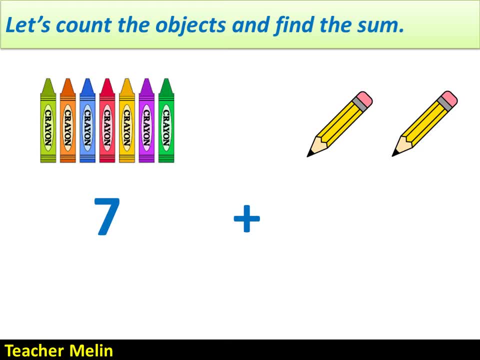 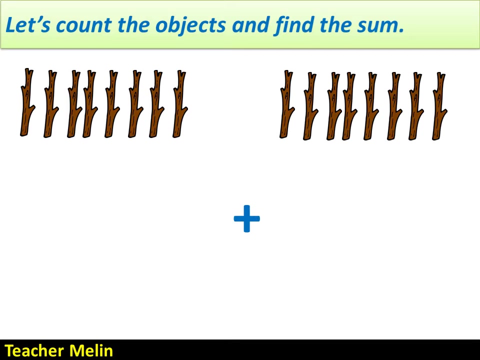 Let's count the pencils: 1, 2, 2 pencils, 7 plus 2. 7 plus 2 equals 9, So there are 7 crayons. There are 9 objects in all. How about this? Let's count the sticks: 1, 2, 3, 4, 5, 6, 7, 8. 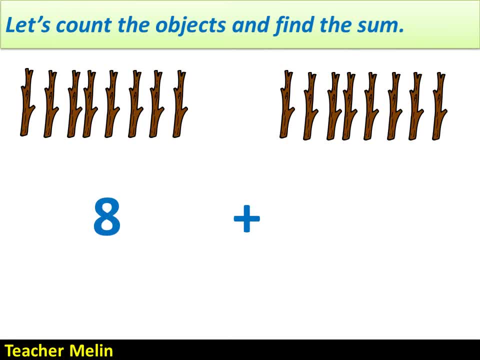 There are 8 sticks on the first set, Another one: 1,, 2,, 3,, 4,, 5,, 6,, 7, 8. There are 8 sticks on the first set. There are also 8 sticks, 8 plus 8. 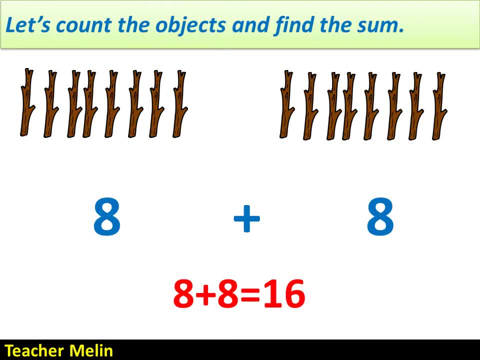 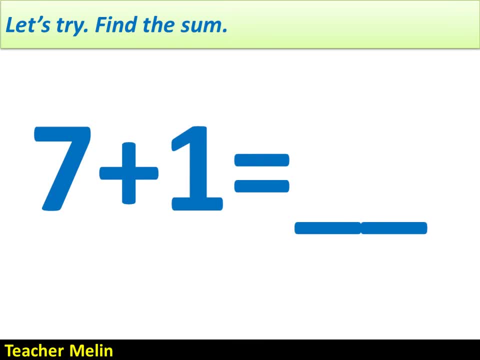 8 plus 8 equals 16, So there are 16 sticks in all. Let's try Find the sum. 7 plus 1 equals. What is the answer? The correct answer is 8. 7 plus 1 equals 7. 7 plus 1 equals 7. 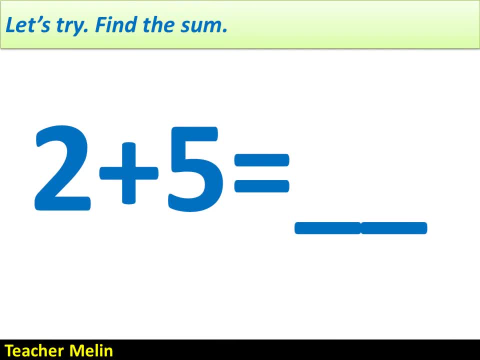 7 plus 1 equals 8. 2 plus 5 equals. What is the correct answer? The answer is 7: 2 plus 5 equals 7. 1 plus 9 equals. What is the correct answer? The answer is 10: 1 plus 9 equals 10.